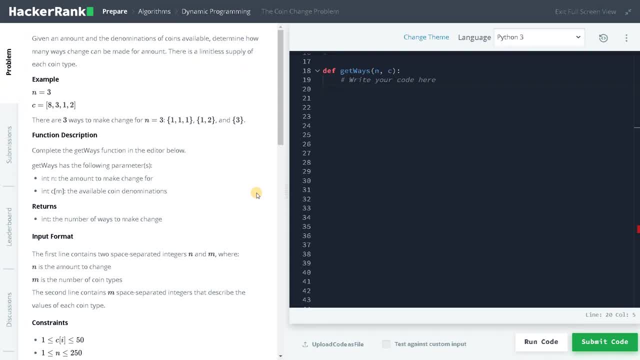 hello everyone. this is ashwin here, so it's been a long time. i have posted, uh, some videos, so i'm going to start it again and i'm going to touch on dynamic programming, which is the last part of the playlist. today we are going to solve the coin change problem. 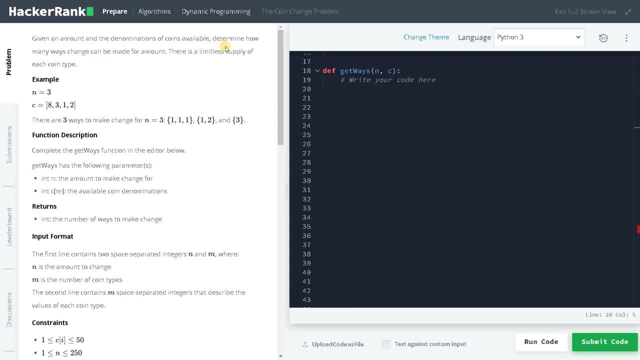 given an amount, and the denominations of coins available determine how many ways change can be made. for amount. there is a limitless supply of each coin type, so this is one condition. we have to keep it in mind while creating the logic. so let's see an example here. 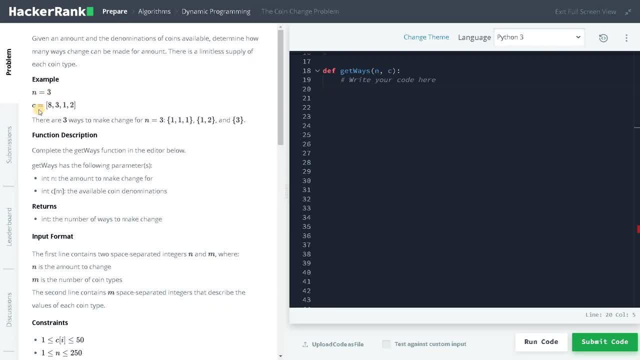 so here we have to get the change for three. so this is the list of coins, which is a length of four. so you can get the coins in like, we can have it as like three and we can have one one, one as like another combination and we can have one plus two. so the total number of ways to get the change. 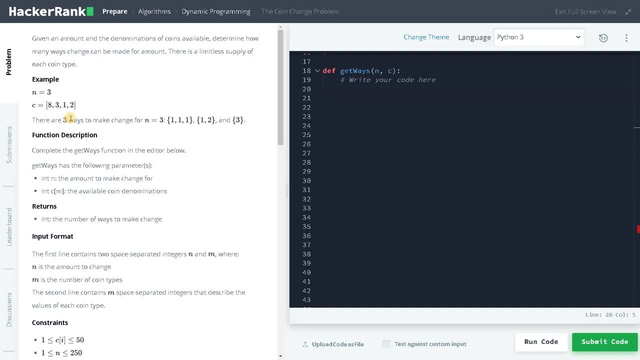 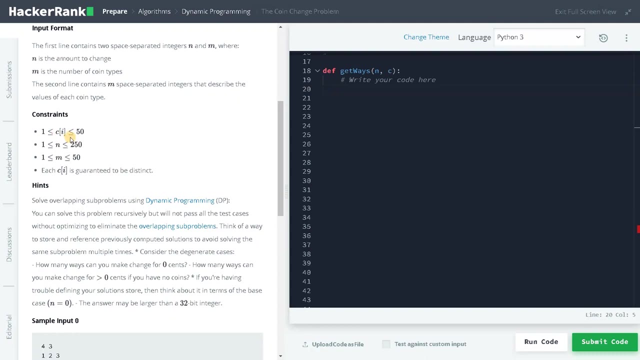 for three is three. so like this we have to produce the output. but if you try to solve it in like, using a brute force approach, it will definitely exceed the time limit. let's also check the constraints here. you can see the coin range is in the range of like. 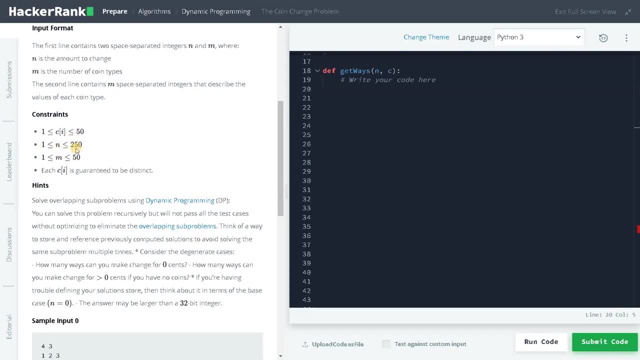 1 to 50 and yen is in the range of like 250 and yum it's in the range of 50. so if you try to get the change from this list means it will definitely, uh, go out of the time limit, so we have to use. 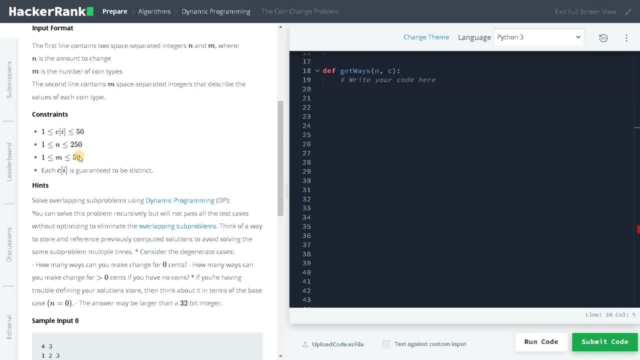 dynamic programming to solve the sub problems and keep it in some memory. so here also they have mentioned think of a way to store and reference previously computed solutions to avoid solving the same sub problem multiple times. so this is the main core part of the logic we have to follow. 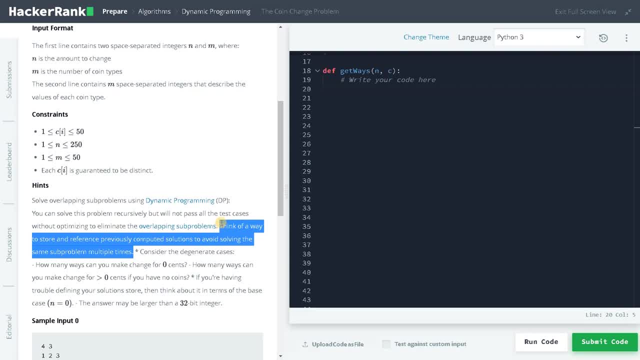 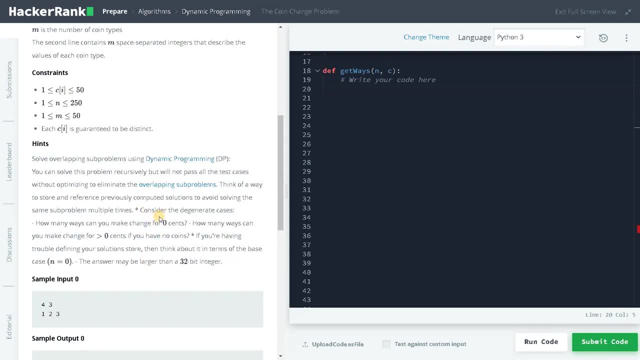 this approach will help in many dynamic programming problems. even in some complex problem you could solve using this dp approach. so here also they have mentioned some example. like we can define some base case and keep on incrementing for other cases. so usually the dynamic programming will be. 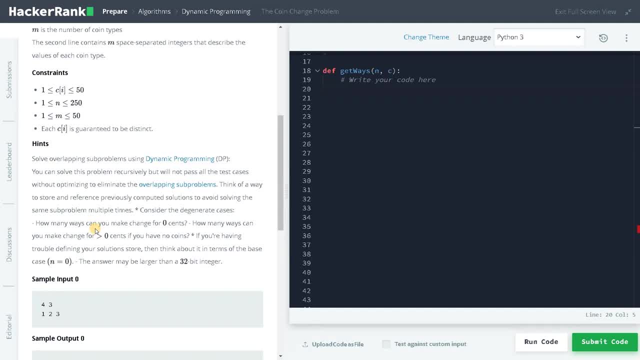 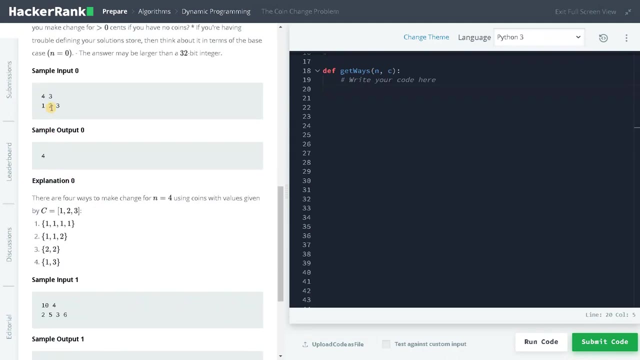 combined with, like a recursion or iteration by storing it, some arrays or multi-dimensional array. so here also we are going to store the previous computed values in an array. i will show you with an example: uh after uh doing the coding, uh, so this is another input. so the change we have to get is four and the number. 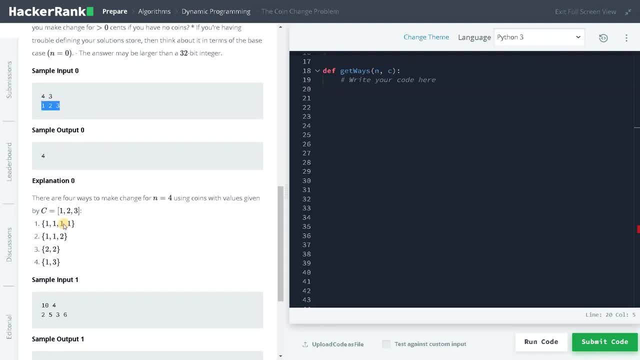 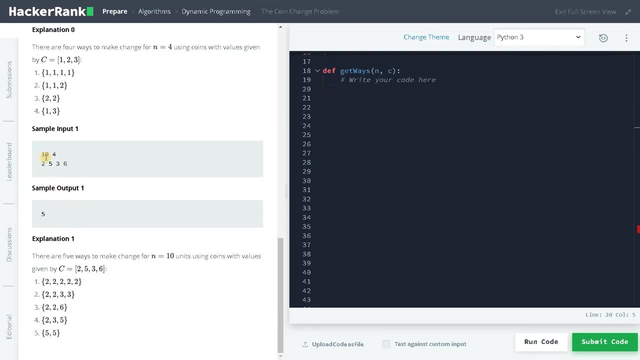 of points is three. so we have one, two, three, and here they have mentioned, uh, all the possible ways that we can get the change, and this is another input, and these are the uh coins, and here we have like five ways to uh produce the uh change. now let's dive into the logic. 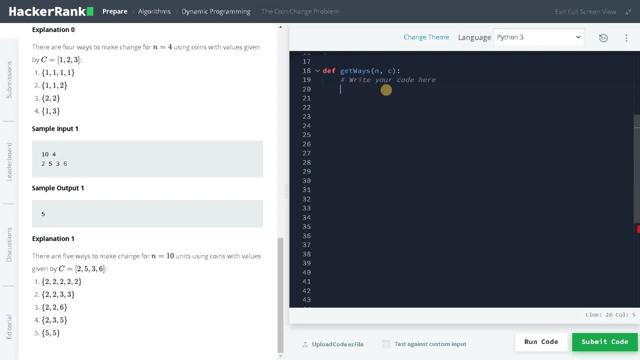 i'm going to use the recursion approach method. uh, in this i'm going to solve it using, uh, iterative approach. so iterative approach, if you guys solve it using recursion approach, means please leave a comment below so it will be helpful for others. uh, as i said, we are going to store the solution in 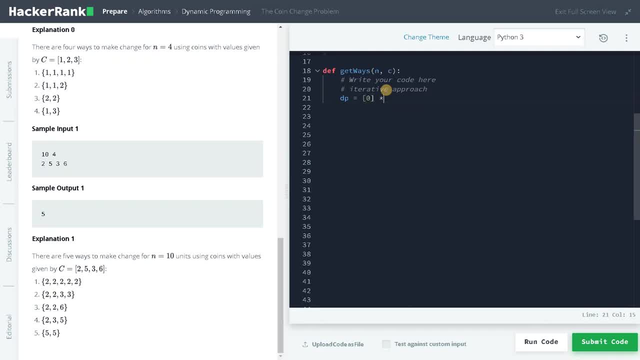 some memory, so i'm going to call it as dp multiplies n plus one. So if you want to solve for a change of one, and let's say if you want to get the result for one means, that result will be stored in this array, in that particular index. 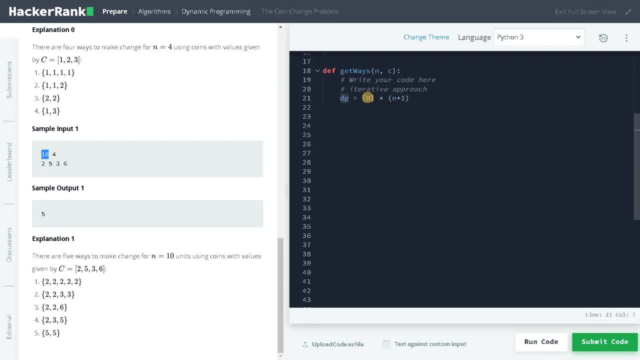 So if we take 10 means if you want to access 10th index, it will be out of it if you just have only n. So that's why I'm just having n plus one. So if you consider here, n is 10.. 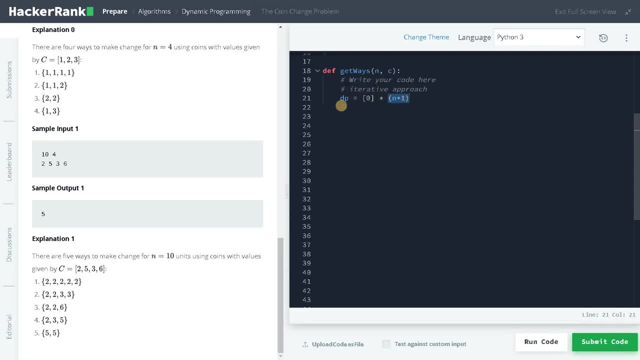 So this will be like 11. So we could access 10th index. I guess that you guys can understand why I'm using this. So most of the problems we'll be using like this only And again the base case- So base case will be: dp of zero- is one. 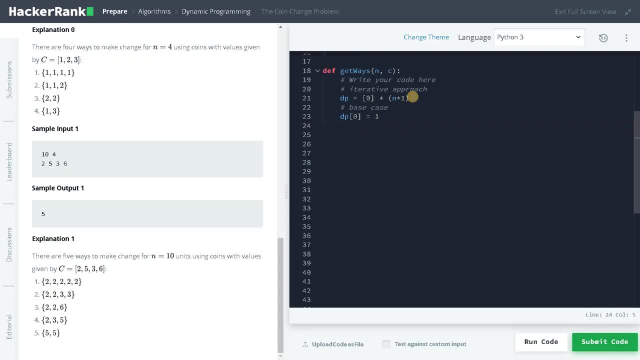 So using this only, we are going to iteratively solve the sub problem And this will be the main logic. So for in range of lenox Of C, I'm just iterating through the coins for J, in range of C of five, two n plus one. 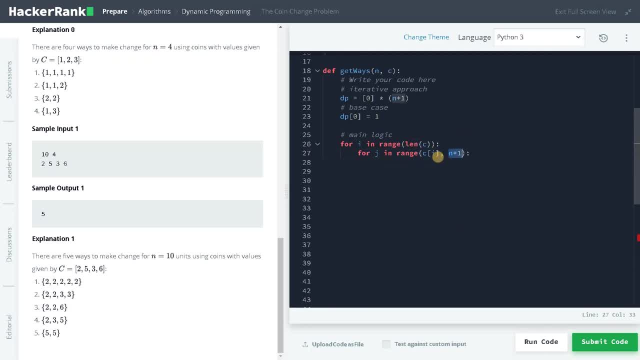 So this is the length of the DP And I'm just starting the loop based on the coin value. So here if the coin value is two means it will go up from two to 10.. So I am gonna update the logic so DP of J plus equals DP of J minus C of I, and I will also print: 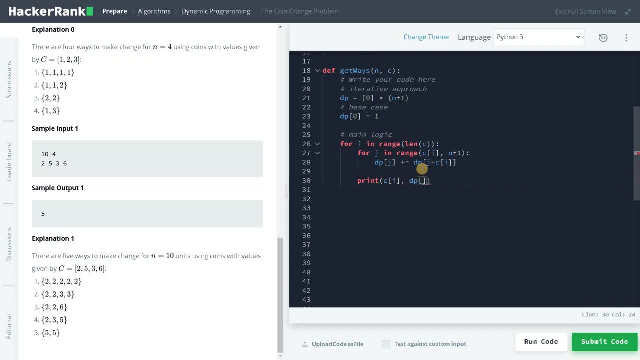 C of I and DP of I- sorry, just DP, just to show how it is changing And we can, and we can easily see how the problem is solving itself, like by using the previous computation. So, finally, I'll just return DP of n, which will have the final solution. 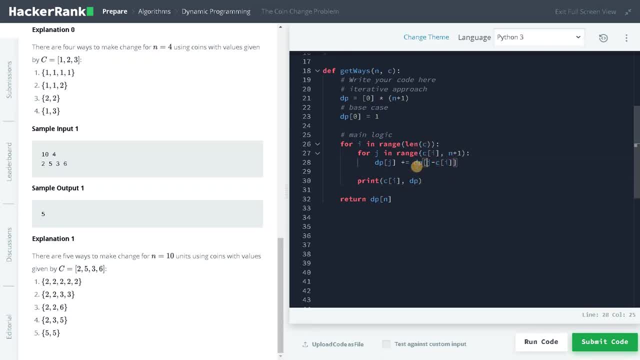 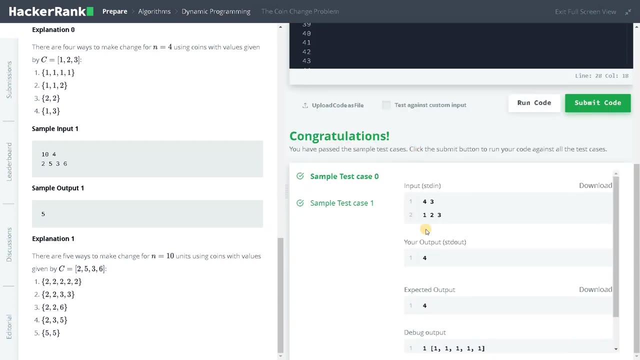 Okay, so this logic I'm just subtracting from the index with the coin value, So it will be just updating to the DP of J, So let's run the code once. Okay, now you guys can see the debug output, So let's run the code once. 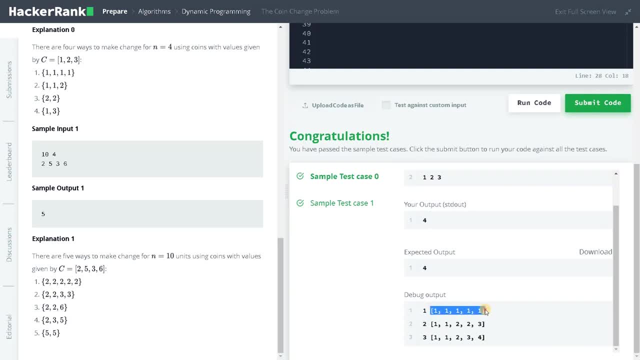 Okay, now you guys can see the debug output. So let's run the code once. Okay, now you guys can see the debug output. So this is the coin value and this is the array. Initially, the array will look like this initial array: DP equals what is the 123. 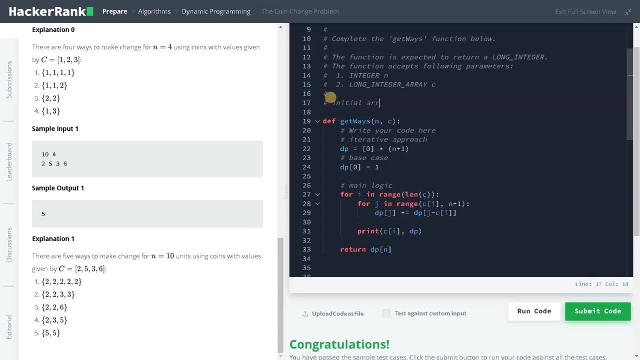 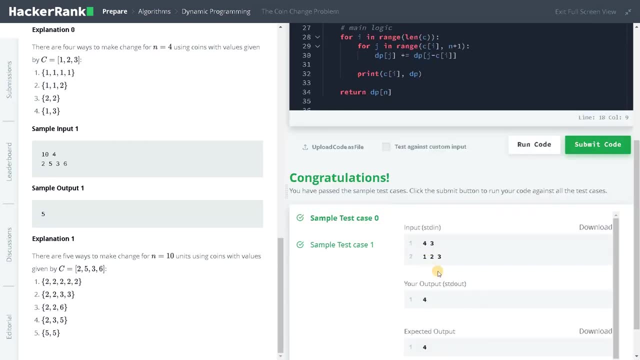 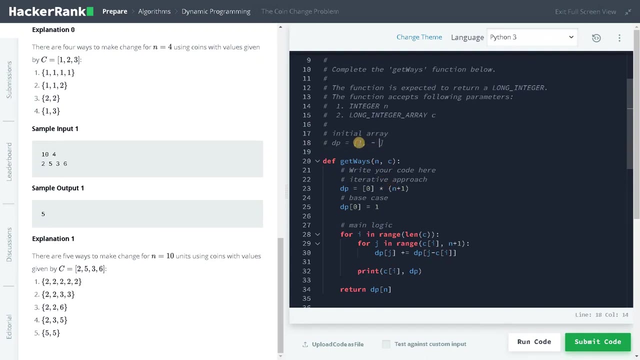 Initially the array will look like this initial array: DP equals what is the 123.. So we'll be having like four index: one zero, zero, zero and zero. So we'll be having like four index: one zero, zero, zero and zero. 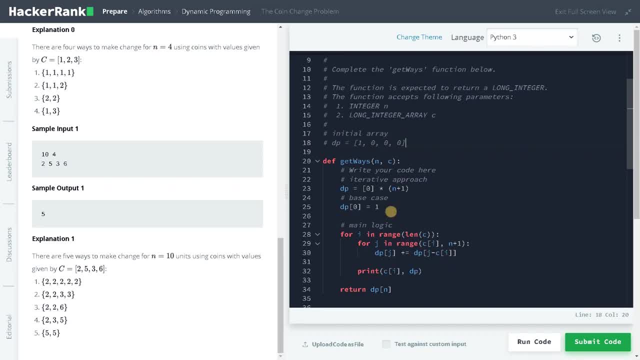 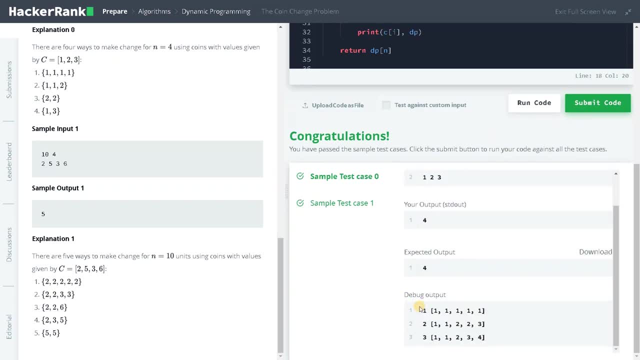 Okay, so this is the DP initialization. Now we will see the debug output. So first we are solving the sub problem. So first we are just taking only one. So if the change we have to give is only one means we are just updating the values based on it. 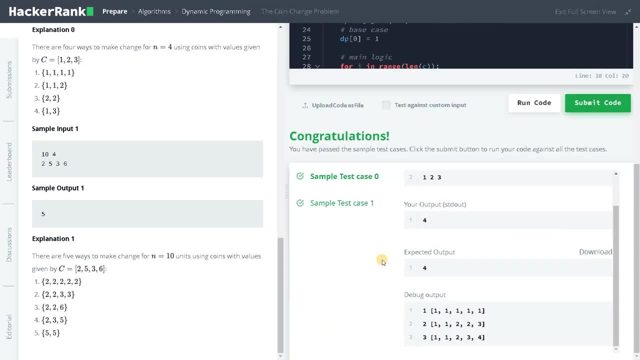 So, as I already said, okay, for the first, we have only one coin, that is one, and the change we have to get is four. So initially this will be one and everything else will be zero. And based on this expression, okay, based on this expression, so j minus c of i, so that 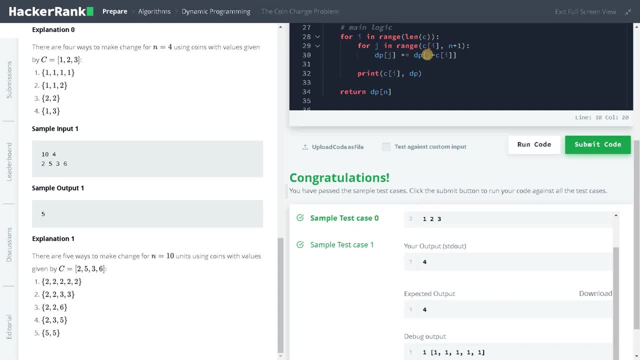 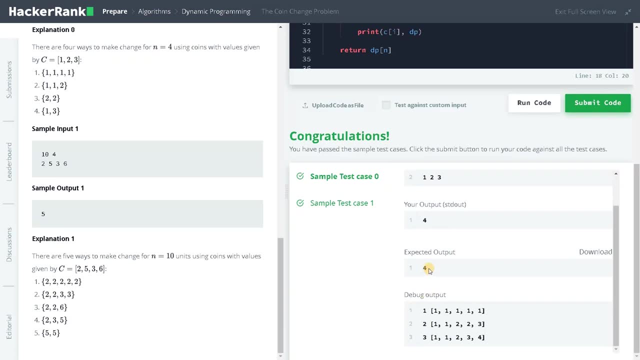 will be one minus one, and it will be updated. And again it will go to two minus one, And again this will be updated and it will be just keep on appending. So to get the change four Using only one coin, that is one. the number of ways is one. 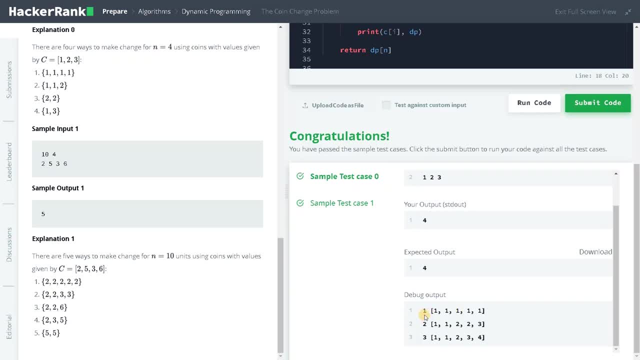 So this is the sub problem. Let's go into the next iteration. So we have the coins one and two and we have to get this change, that is four. Okay, now again. so, using the same logic, we will be just adding, so it will be starting from two, based on the coin index. 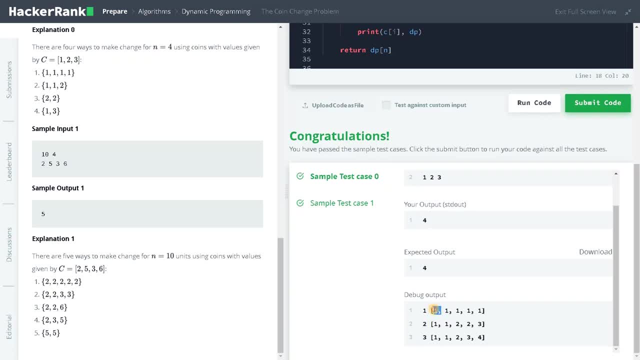 And if you consider the previous one, so one, One plus one, it will be two, And again one plus one. again this will be two, and one plus two is three. So finally, we are getting the result for the another sub problem. 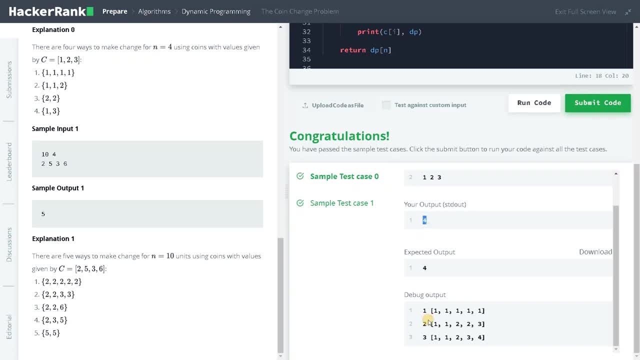 That is for the change, four with only two coins, one and two. the number of ways we can arrange is three. I guess you know the possible arrangements right, So So this will be like one plus one plus one plus one, that is four ones. 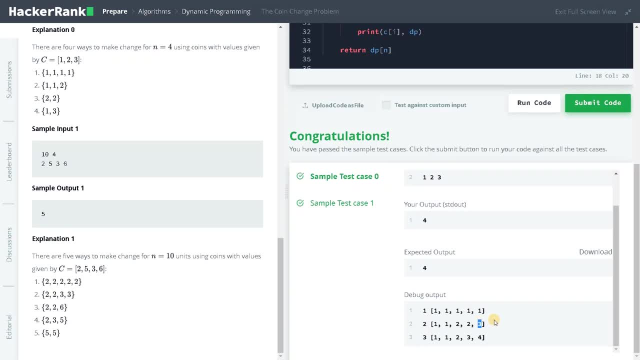 And for this we have one plus one plus two. that is again four. two plus two is again four. So the total number of ways we can get this four is three, And again we are considering three coins here. Now, using the previous array, we will be updating the logic starting from third index. 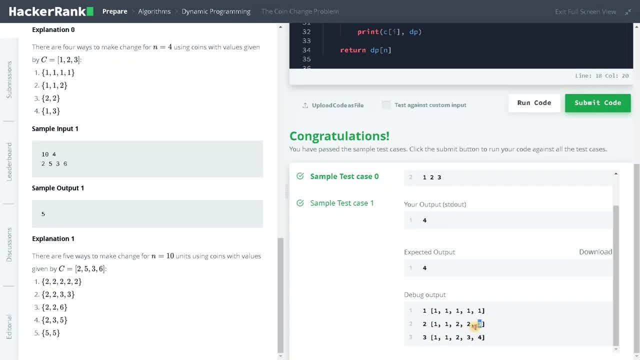 So two plus one is three, And three plus one is four. So Three plus one is three. So the number of ways is four. Like that, we will be just keep on solving the subproblem until we reach the final solution. So finally, we are just returning DP of n, which is this: four.